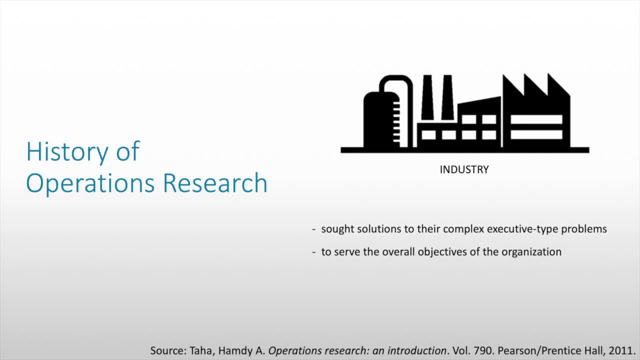 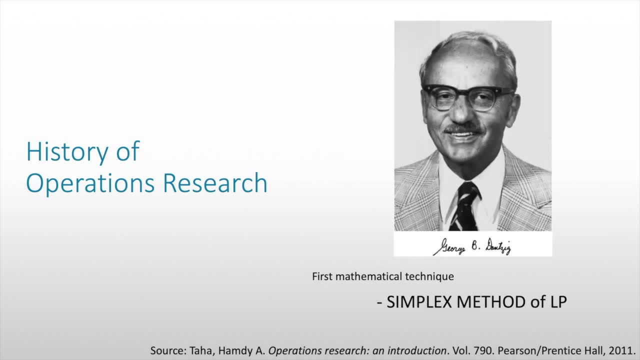 complex executive type problems to serve the overall objectives of their organizations and utilization of the effective tools. The first mathematical technique in operations research is called the simplex method of the linear programming. This was created by George B Danzig in his PhD thesis. To give you a little story, while George B Danzig was a PhD, 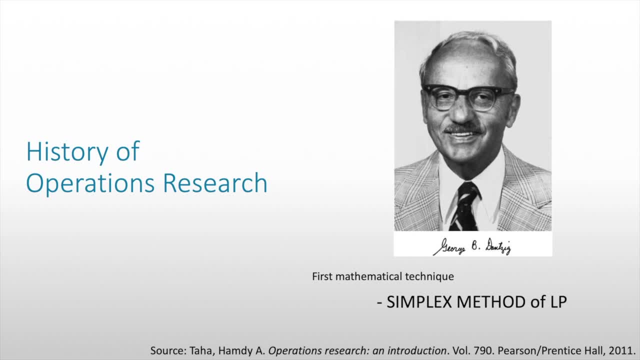 student. he came in late to one of his classes. As he came in he saw different problems that was written by his professor on the board and he thought these are his homeworks. He wrote them all down and then by the next meeting he answered two, if I'm not mistaken, out of the three problems. 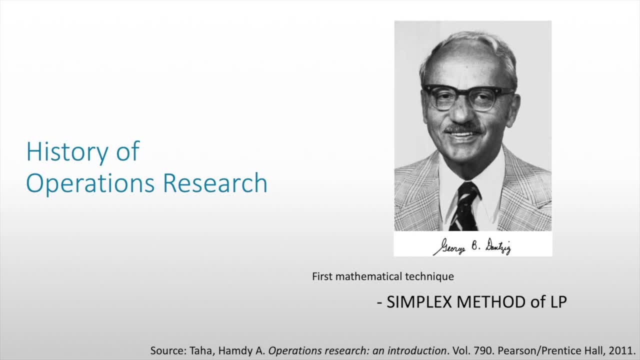 But then he didn't realize that these are actually not the homeworks, but these are actually mathematical problems which have not been solved yet, And when his professor or his advisor saw these, they realized that he was able to come up with one of the best solutions in solving linear. 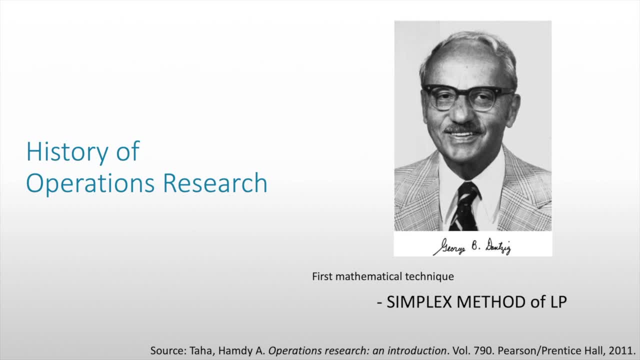 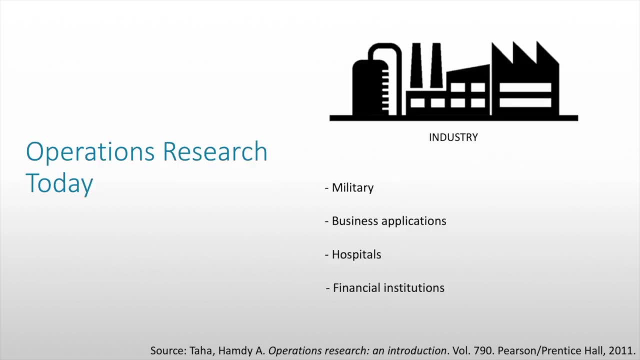 programs, and that is the simplex method. And then these homeworks became his dissertation or his PhD thesis. Operations research today is not only used by military, but also been used in business, hospitals, in financial institutions, libraries, city planning, transportation systems and even 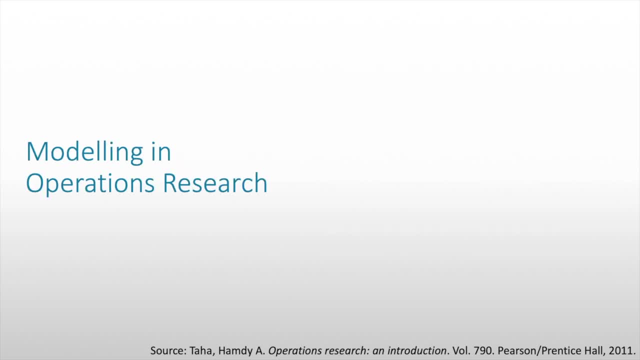 crime investigations. So what are the different models in operations research? First, we have iconic models. Iconic models are basically prototypes or real-life samples of what the real-life problem is, For example, a toy plane. A toy plane is an iconic model of the real plane. 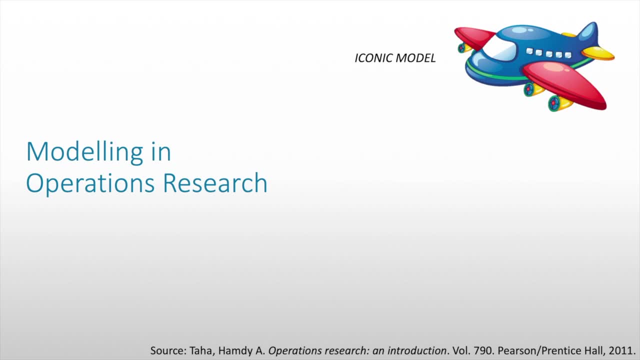 which is a very big one, And since we wanted only to play on a smaller version, then we create a toy plane. This is an iconic model. Another model is the analog models. Analog models are kind of abstract representation of a real 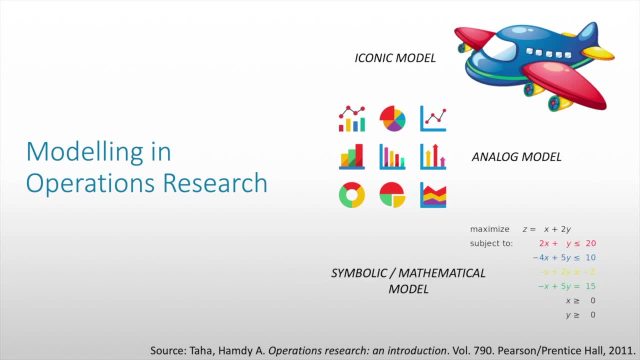 system, For example graphs, And then we have symbolic or mathematical model. An LP or a linear program which is written here is an example of a mathematical model. It basically models the real system through mathematical models. And then we have symbolic or mathematical models, And then 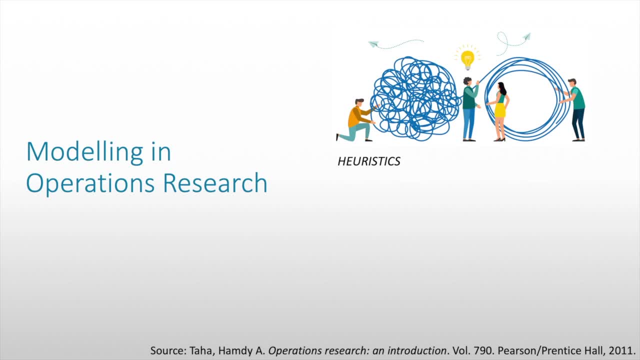 we have diretrical equations And then we have mathematical functions. Then, with advancement of technology, there are two other models which have been created. currently. One is heuristics and the other one is simulation. Heuristics is basically rule of thumb or other techniques which have not 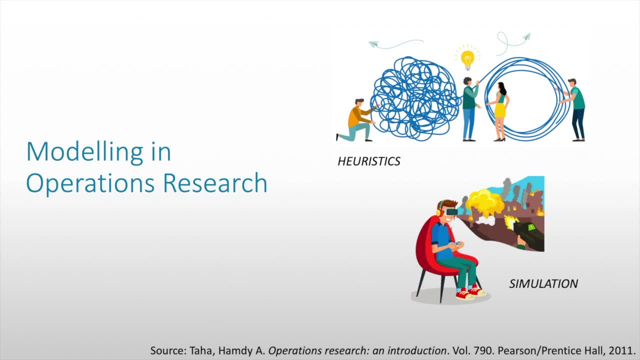 been used before and may be used or may be useful in the future. Those are heuristics. For example, in different problems on scheduling, one heuristic would be to schedule those with shortest processing time. That is a heuristic. Then simulation models are digital. 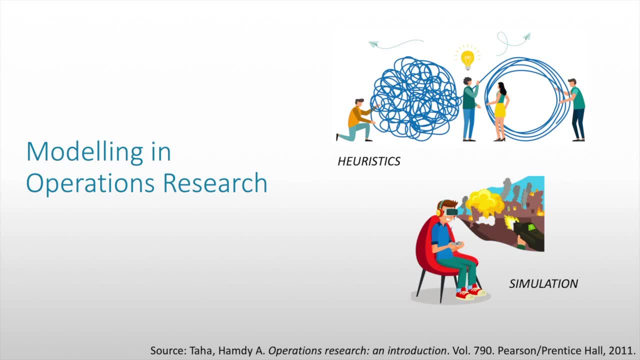 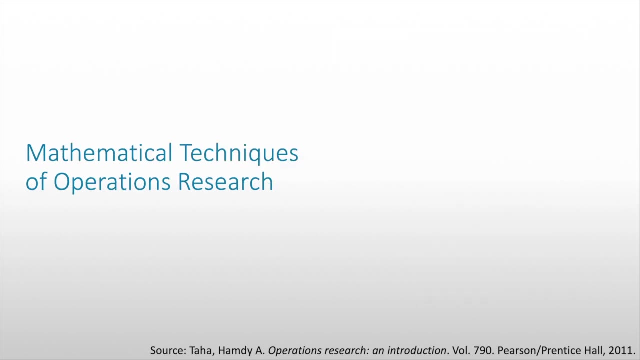 representations which imitate the behavior of a system using a digital computer. The statistics describing the different measures of performance of the system are accumulated as the simulator advances on the computer. So what are the mathematical techniques for operations, research? We have the following: Linear programming, or LP. Then we also have dynamic programming. 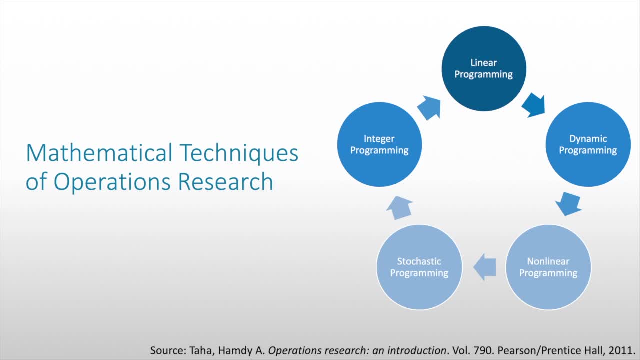 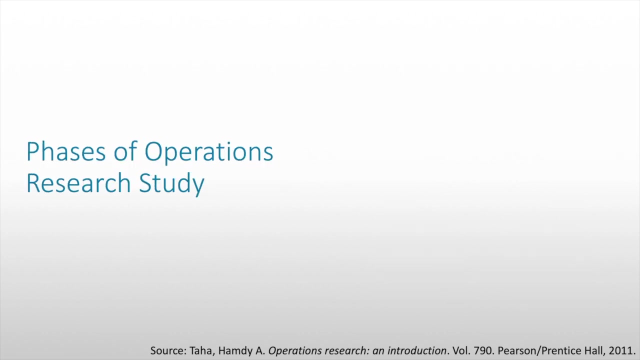 Then we have non-linear programming, stochastic programming and also integer programming. As we go through our different lectures, we will be talking about each one of them in depth. For now, we will focus on linear programming. So what are the different phases in order to do operations? 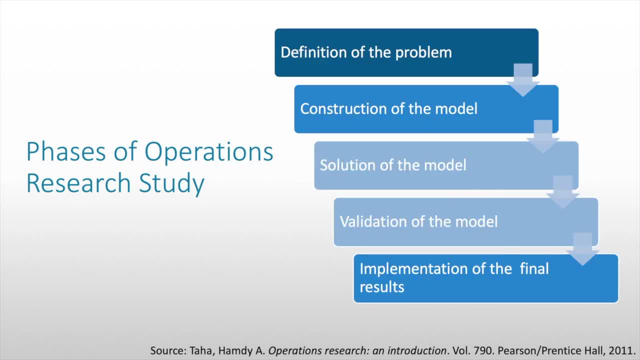 research study. First, we have to define the problem. This is very crucial and very critical. We have to understand the problem at its core in order for us to know what we want to solve and know what kind of problems we will encounter in the future. Then we have 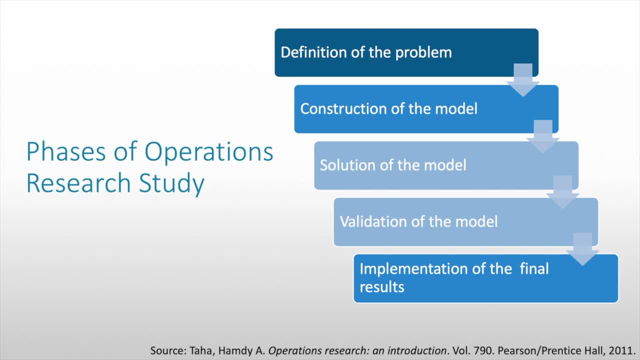 the construction of the model. This is the part where we're going to use mathematical models in order to replicate our real system. So this is the part where we construct our linear program or our integer program. Then we have the solution of the model- This part. 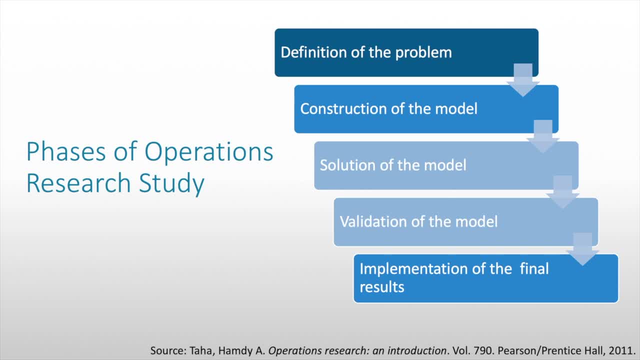 is basically solving our model that we constructed from the previous stage. Then we have the validation of the model. Validation of the model is basically to validate if our solution to the model is actually correct. This is basically done through implementing our solution to a prototype. 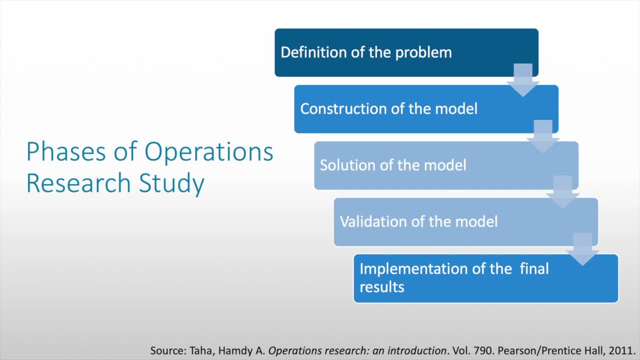 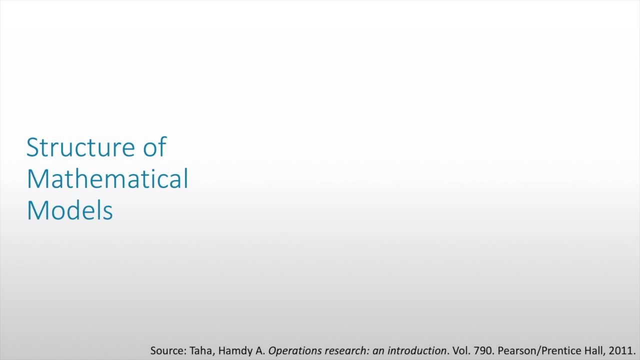 system. Then we have the implementation of the final results, where we have to implement our solutions to the real system. Now we will talk about the structure of mathematical models. This is an example of a linear program, and a linear program is composed of the following: 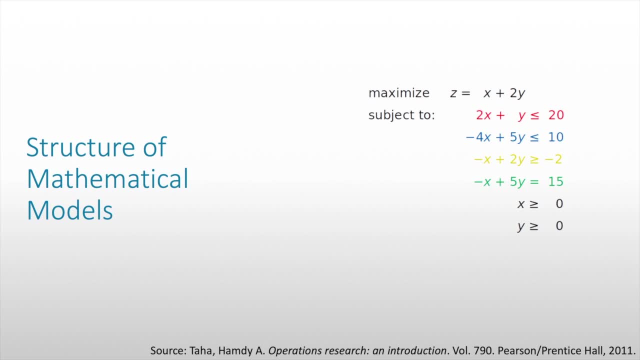 elements. Each element will be explained individually on the part of the model, Part 2 of our lecture. First we have the objective function, Then we have decision variables And then the different parameters and the different constraints. Again, we have an objective function, we have decision variables, we have the different parameters and then 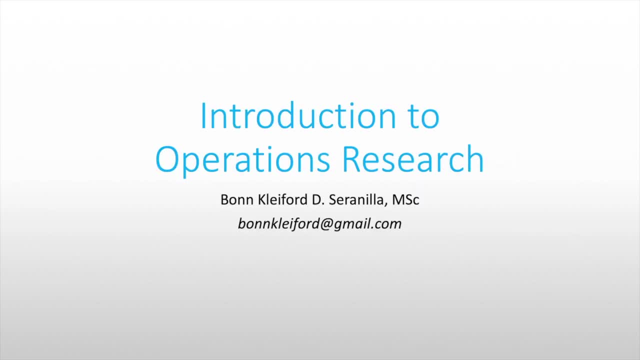 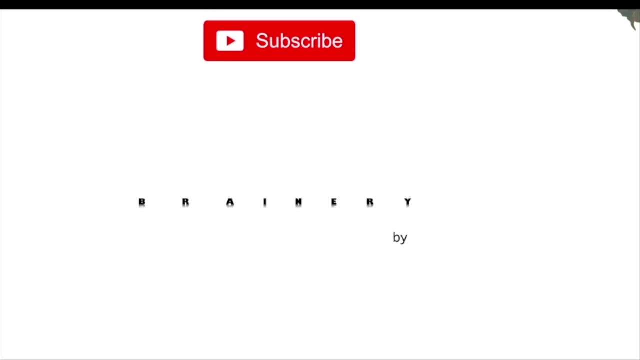 the set of constraints. So that ends our lecture for today. Tune in for the part 2.. This is Bonkli for DC Uranelia. Thank you very much for watching. Transcription by ESO. Translation by —. 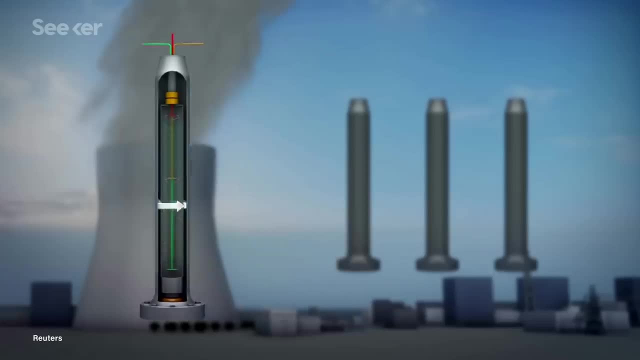 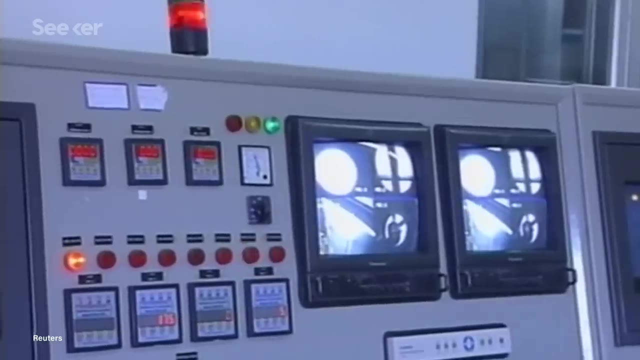 Nuclear programs are constantly in the news, with reports that they're enriching uranium. Usually the stories mention percentages and centrifuges, but to the uninitiated it's not clear why these things are important. What exactly does it mean to enrich uranium? 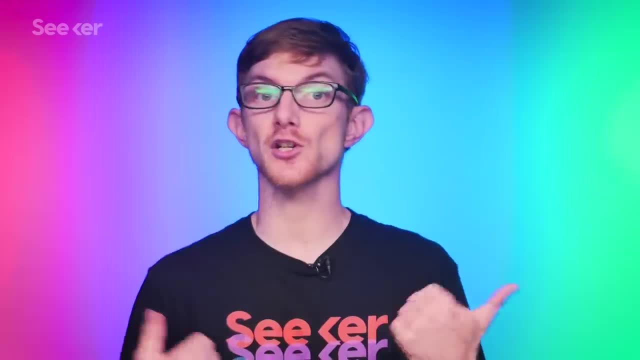 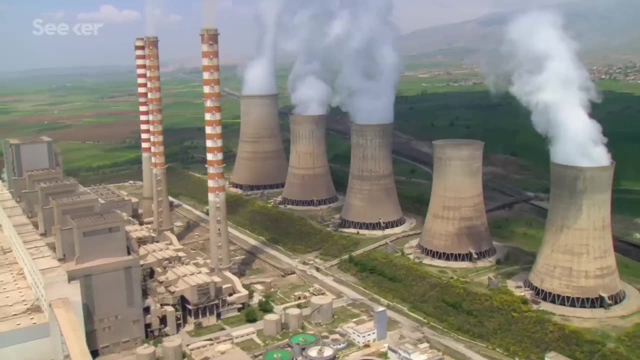 And at what point should we be worried? Now, when I imagine enriching uranium, I picture teaching uranium to paint or dance or something. but I looked it up and that's not what it is For nuclear power or weapons. the isotope of 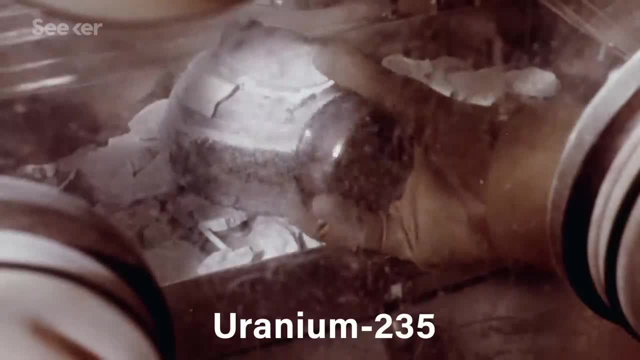 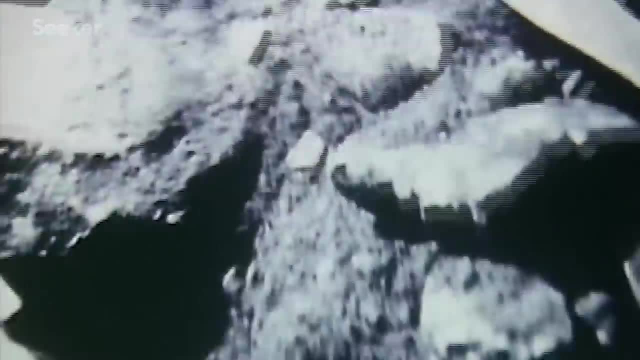 uranium we're after is U-235,, which has 92 protons and 143 neutrons, But the vast majority of uranium we pull out of mines- 99.3% of it- is the isotope U-238,, which has 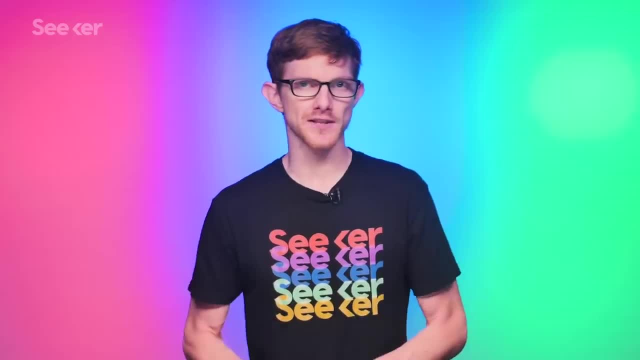 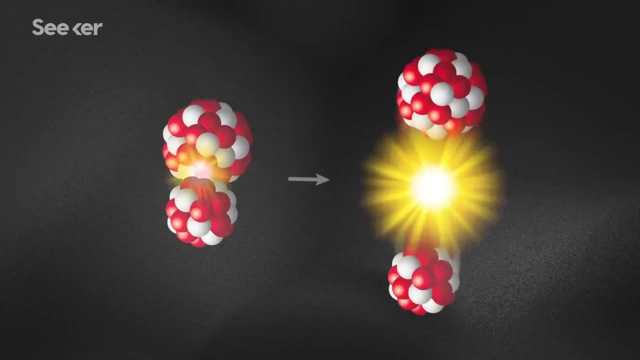 three more neutrons and behaves differently. Only about 0.7% of uranium in the world is U-235.. U-235 is fissile, meaning all you need to do to split it is hit it with a low-energy thermal neutron. The neutron doesn't smash the nucleus apart, but instead is absorbed. 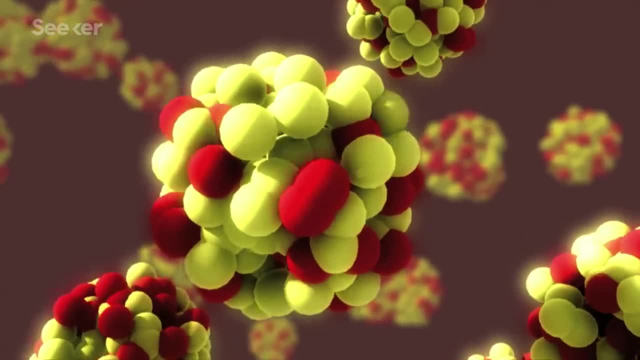 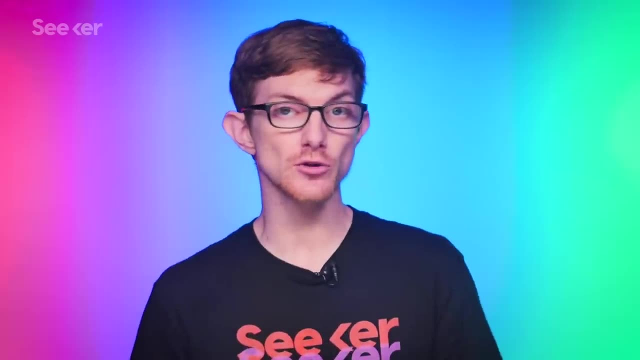 by the atom, making it unstable. When it splits, it releases energy and more neutrons that can then repeat the reaction with other U-235 atoms. You can still split U-238 atoms, but you need high-energy neutrons to do it, which is less efficient. While nuclear bombs that want to release a lot of energy all at once have concentrations as high as 90% U-235.. The challenge is: how do you take naturally occurring uranium, that's 0.7% U-235, and up its concentration to those lofty numbers?